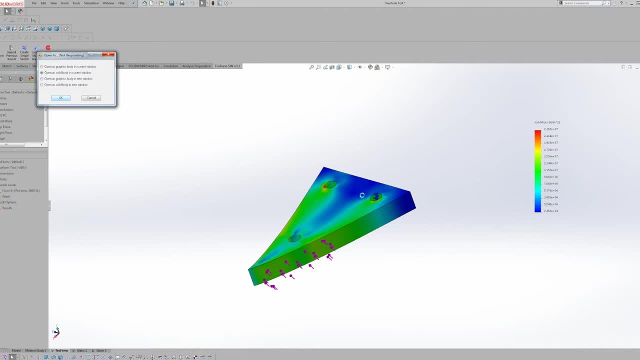 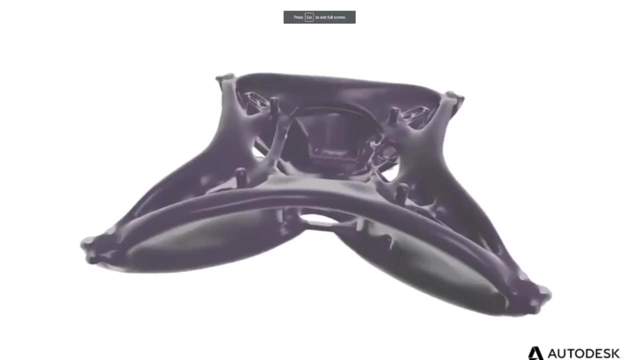 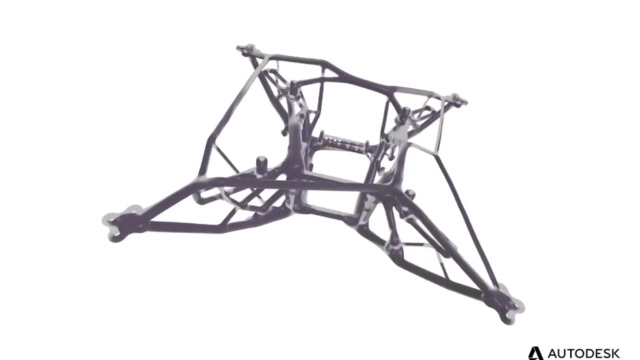 FEA software. Now the difference between this and algorithmic design is that it basically takes the designer out of it once they've specified the boundary conditions. This amazing clip from Autodesk, from their new Fusion 360 generative design plugin, shows the optimisation of a quadricopter chassis and it looks very natural and organic. It almost looks like. 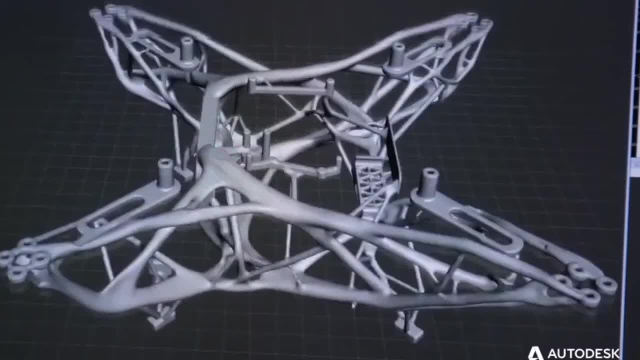 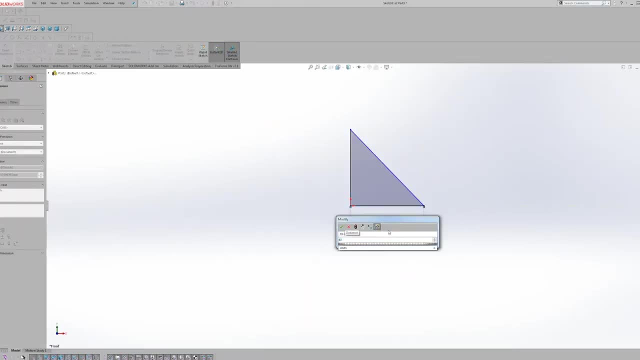 it's evolved to meet the criteria set out in the FEA, And that is, of course, exactly what's happening. This is a little test that I've run with a SOLIDWORKS plugin called Trueform Express from GRM. I created a little flat top cone. 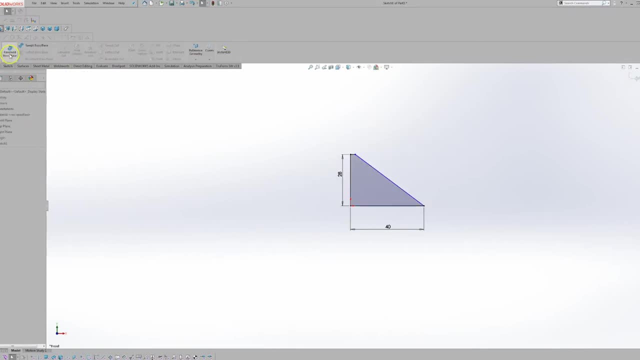 and then run a simulation with a force acting down on the top of it. Now, from there, I tried a number of different things. I ISO clipped it, which is a technique where I can see the maximum stress, And even though that's a great visualisation tool, it doesn't tell. 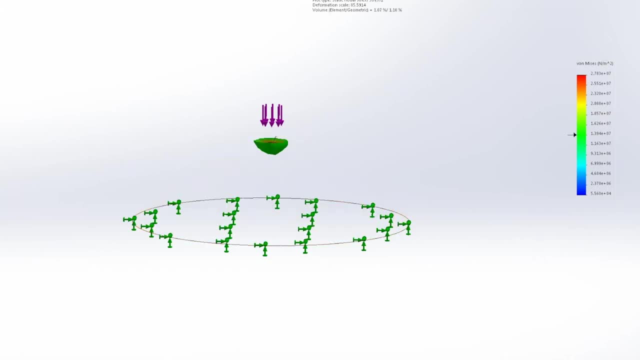 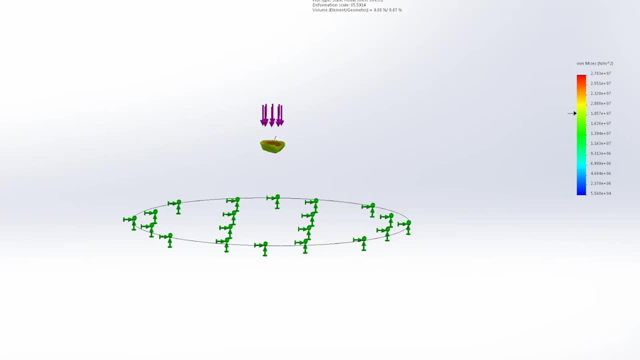 things. I've tried a few different things. I've tried a few different things. I haven't seen anybody that did that. Anyway, as a result, I have a Trueform Optimisation Wizard and it gave me a really strange organic shape which I wouldn't have come up with on my own. 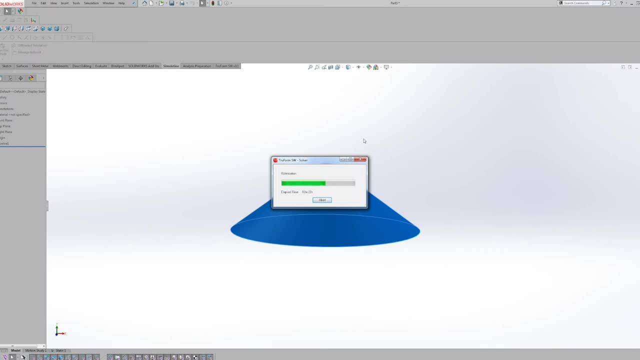 Now, as it happens, this produces an STL which can be 3d printed or manufactured by some additive process, And here we can say there's a massive weight saving. and these kinds of designs are typical of generatively or iteratively or algorithmically generated designs. They 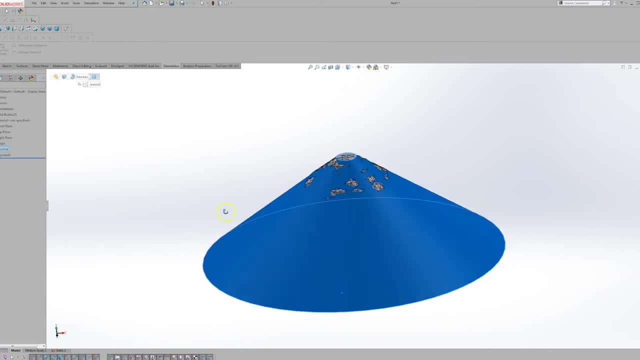 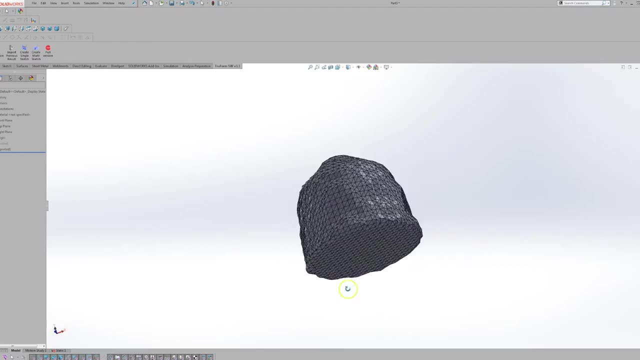 tend to be organic, looking quite strange, looked like maybe bones or a root system that have grown out of nothing. Then you can be manufacture with our additive manufacturing systems. Now Trueform Express actually provides a range of tools in some of their advanced products where you can sketch over the top. 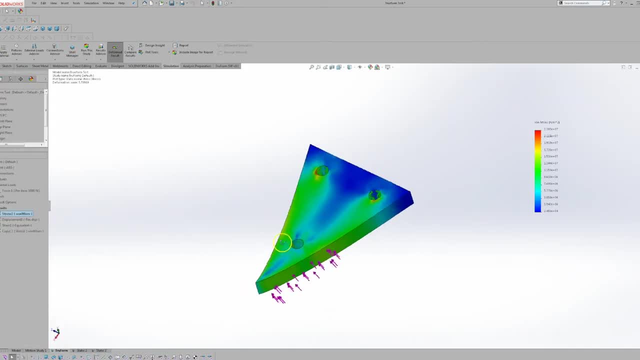 and actually prepare the part for a subtractive process like milling or turning. So this is the result of the optimisation of that super simplified wishbone arrangement that I did an FEA of. Now it's come out with something really organic looking. it's bumpy, it's fairly irregular, but 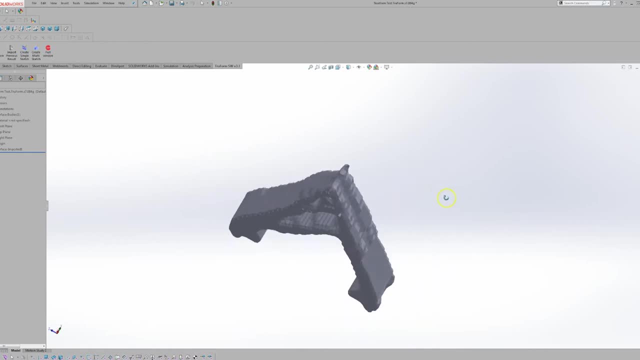 it gives you an idea of the kind of shape that's required to have the perfect optimisation. So underneath you can see there's a little hollow on both sides and also, seeing as I gave it a loading from one side, it's given an asymmetric sort of support network. Now, one thing: it hasn't. 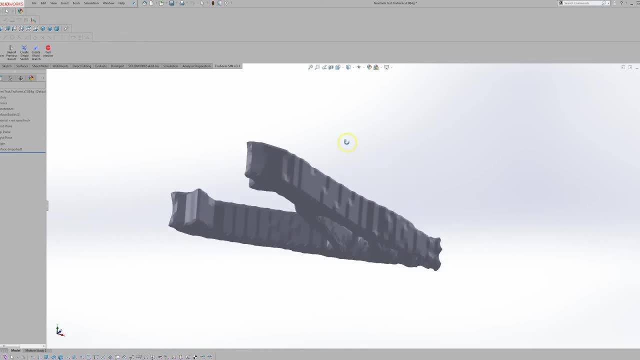 done is it hasn't given support for the back two holes, but that's simply because I specified too greater mass saving in the optimisation criteria. Now I am interested to do this for real for the open RCR wishbone, and we're going to do that in a separate video and I think it'll come out with. 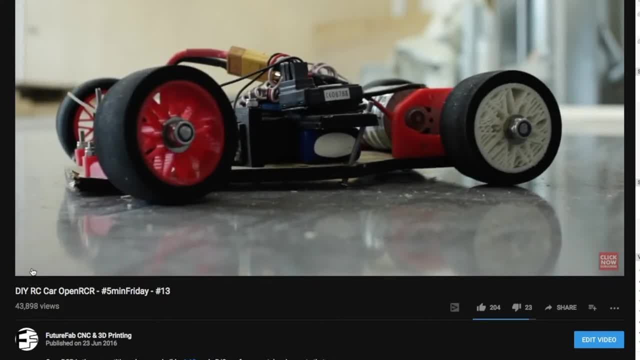 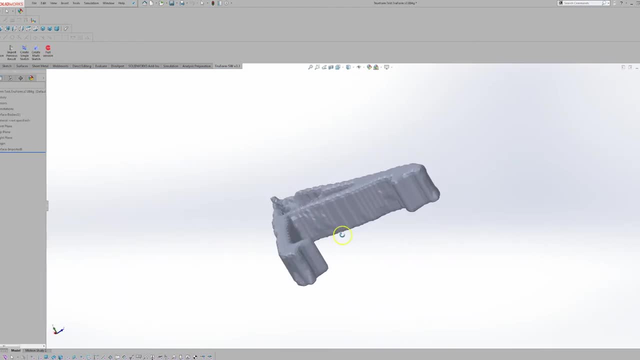 some really interesting and measurable results. But just for the sake of this video, I'm going to 3D print this model and scan it in our hands and see what it actually looks like, because they are quite strange and you can possibly see the reason why this does lend. 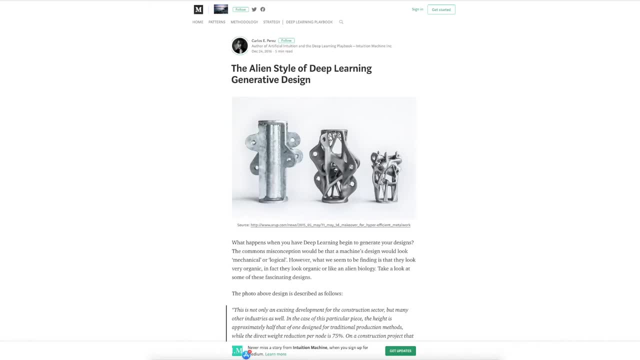 itself better to additive manufacturing. But do keep your eye on this generative design and topological optimisation movement. There's a lot of hype around it at the moment. Here we are. we've got an article called the alien style of deep learning and generative designs- A lot of 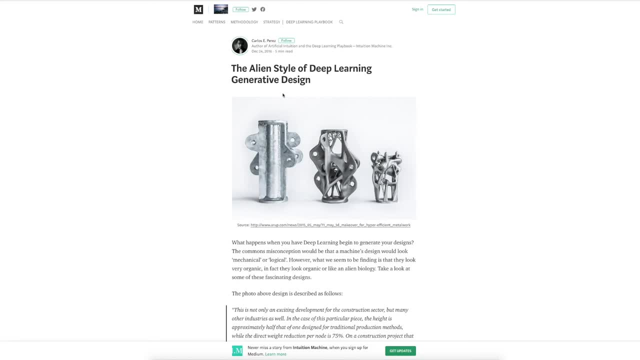 buzzwords. it's linked to evolution and artificial intelligence and machine learning and all kinds of bleeding edge but sometimes irrelevant technologies. It's basically designed by algorithm. It responds to boundary conditions that you give it at the moment. I have no doubt that this could be massive and it will change the face of engineering design, but at the moment 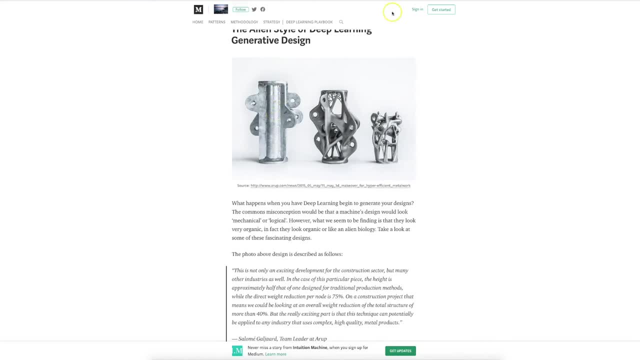 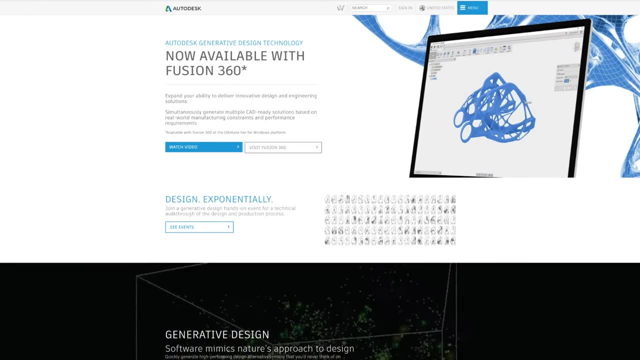 it is just another tool for the design engineer. The thing that I'm looking at the moment is Autodesk Fusion 360 has generative design as a plug-in for their ultimate version. At the moment, it's £75 a month in order to get up to that level, but typically these tools do filter down into 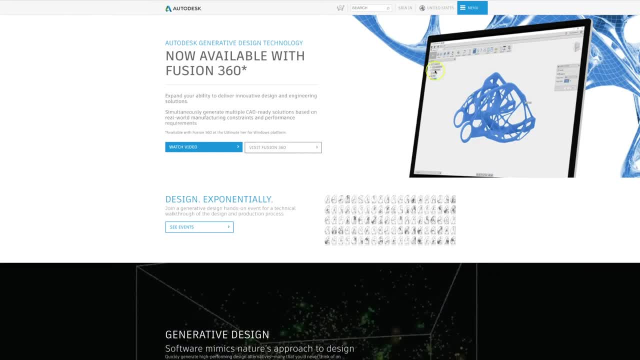 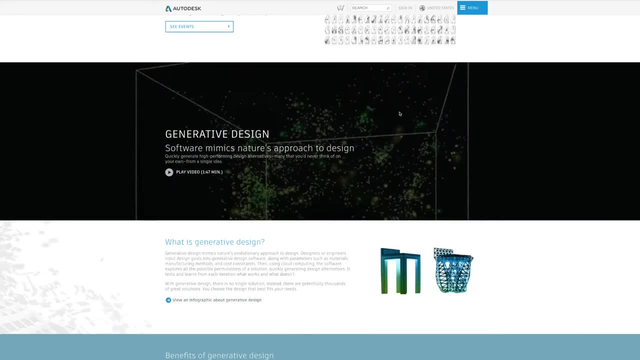 the hobbyist market, and I wouldn't be surprised if this does come along to an affordable price point sometime soon. Similarly, Solidworks has a plug-in in one of their simulation premium, I believe- modules. but we're talking thousands and thousands of pounds. Trueform Express, if you have. 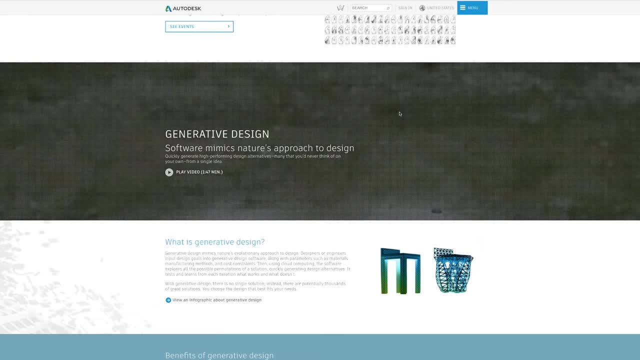 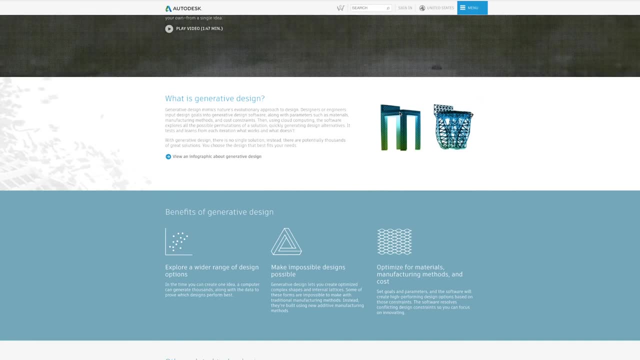 a premium installation is a free download, but it's not cheap to get into. and it's not cheap to get into. It's not hugely stable. but Solid Edge, I have heard, although I have no experience of, is a platform on which generative design is accessible and free, I believe. Do let me know if that's not true, because